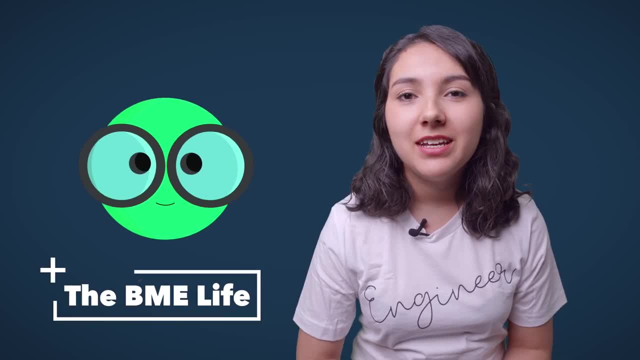 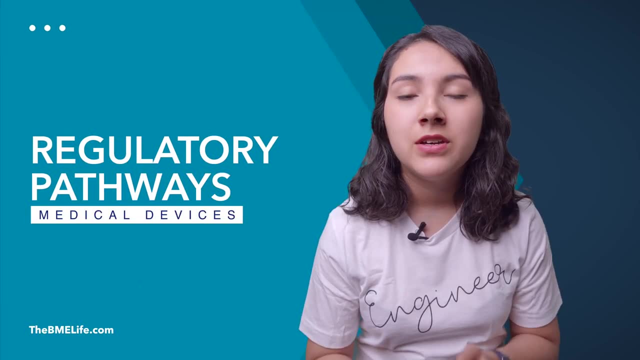 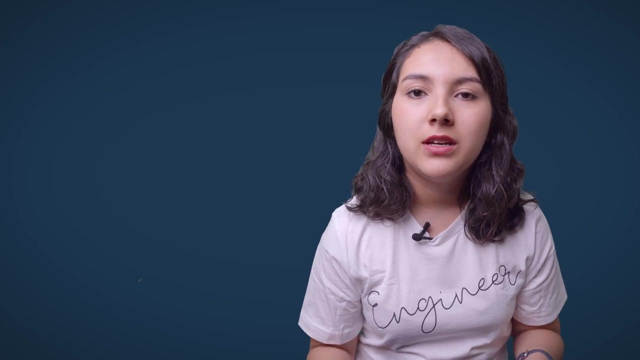 Hey everyone, welcome to the BME Life. My name is Meddy and today we're going to be talking about the different regulatory pathways that the FDA uses to control the approval of medical devices. Usually, before you can market your medical device, it has to be FDA approved or FDA cleared. 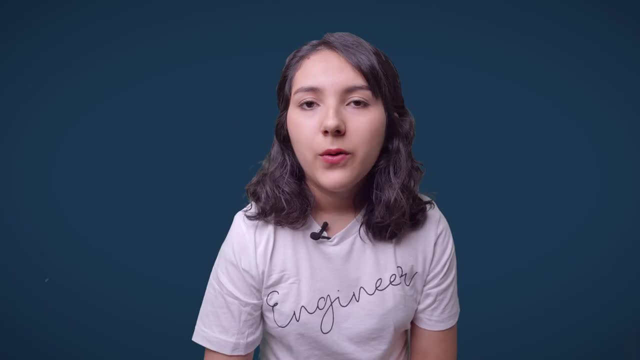 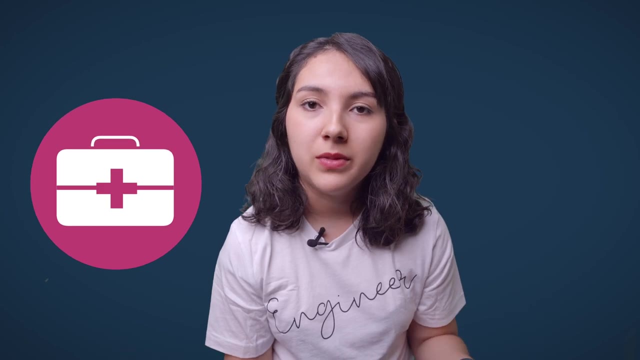 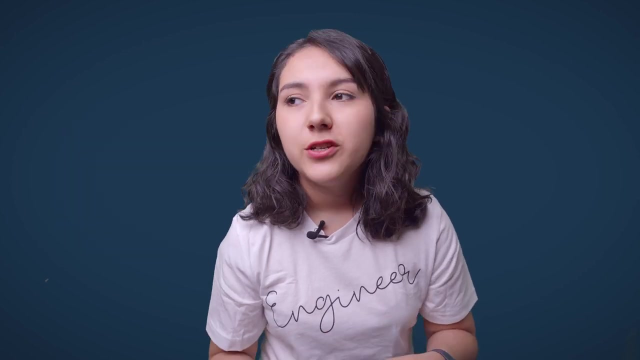 in most cases before you can even sell. So, as you may imagine, there is a very wide range of different medical devices that there can be, and this is why the FDA has several regulatory pathways that you can follow, depending on your device. So, for example, the FDA is not going to. 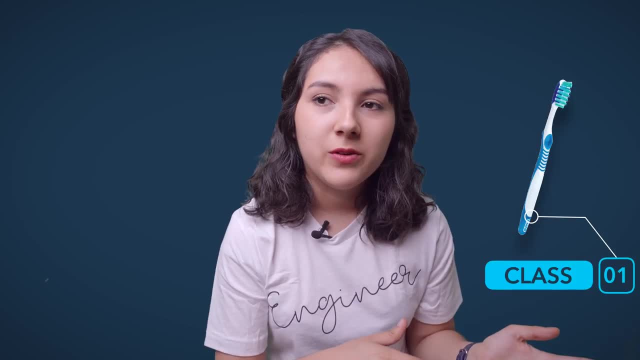 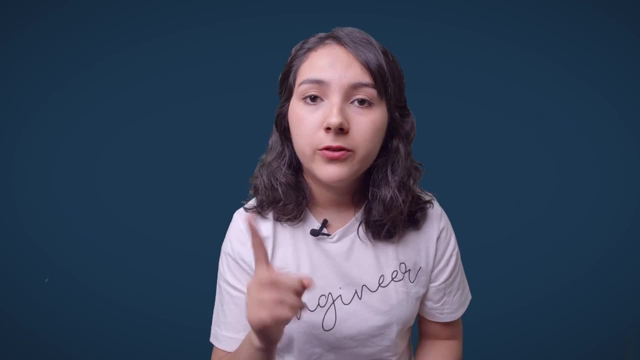 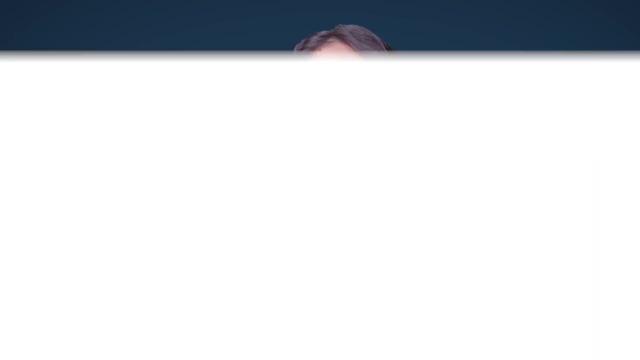 review a toothbrush the same way that it reviews a pacemaker that is implanted near your heart, You know. this is why it's very important to first know the classification of your device. FDA classifies medical devices in three main classes, which are class 1,, 2, and 3.. As the class number increases, so does the risk. 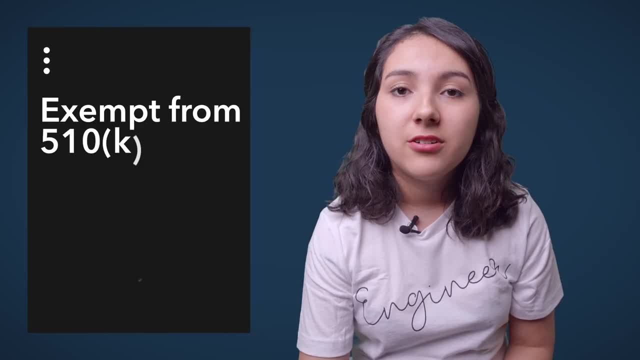 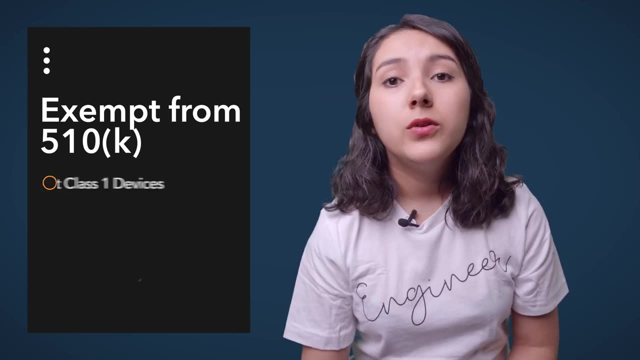 associated with it. There's actually a number of devices that are exempt from having to get a pre-market notification or giving it to the FDA. These include most class 1 medical devices and some class 2 medical devices. So if you're a medical device that has a pre-market notification, 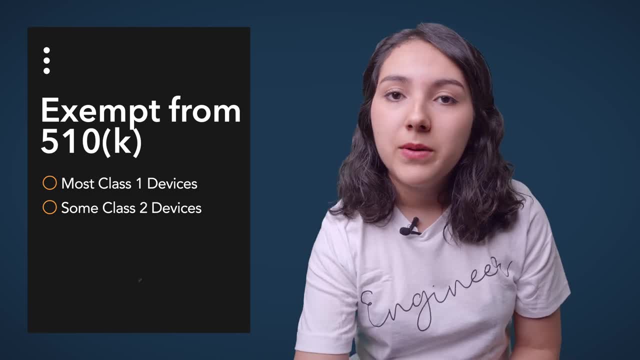 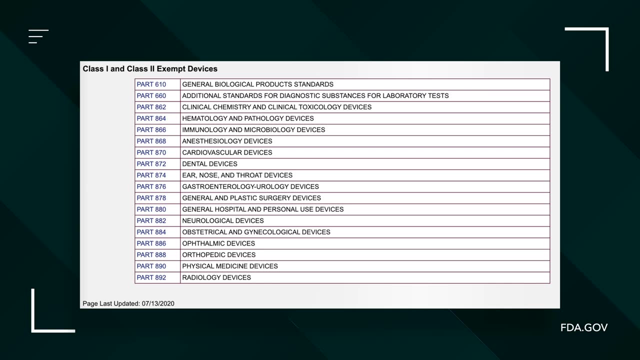 or giving it to the FDA. there's actually a list in the FDA website which I'll link down below. It's FDAgov, But if you go there there's actually a list of the kind of class 1 and 2 devices that. 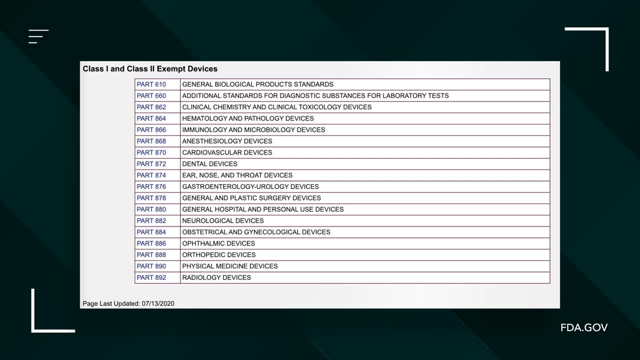 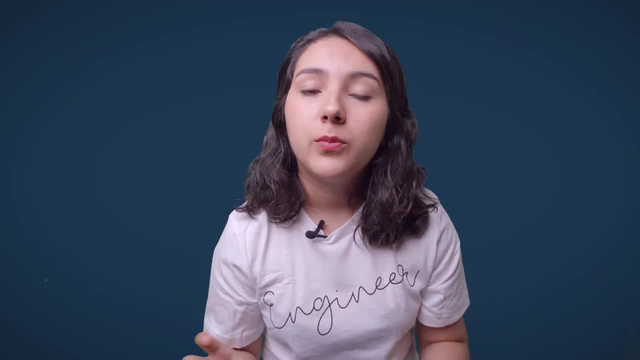 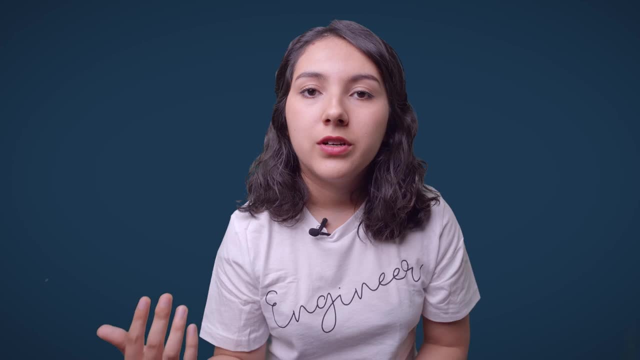 are exempt from having to get any sort of approval or clearance before going into the market. However, even though you don't necessarily need approval or clearance, you do need to register your company and provide your medical device. So if you're a medical device that has a pre-market notification, 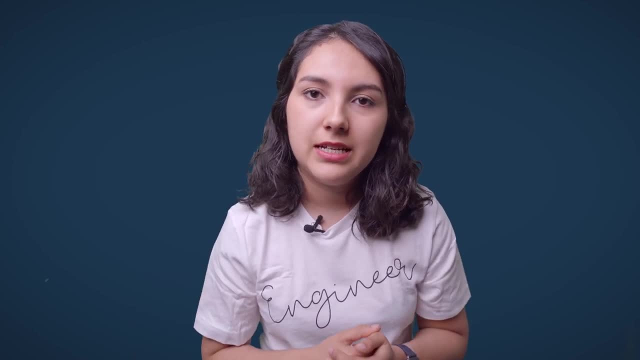 or giving a pre-market notification, go to 510k self- elastic to be able to use it. It's more or less the same specs for any medical device that has a pre-market of 510kusty, or even if you have an injection test or anything like that. They'll come small and the site can possibly. 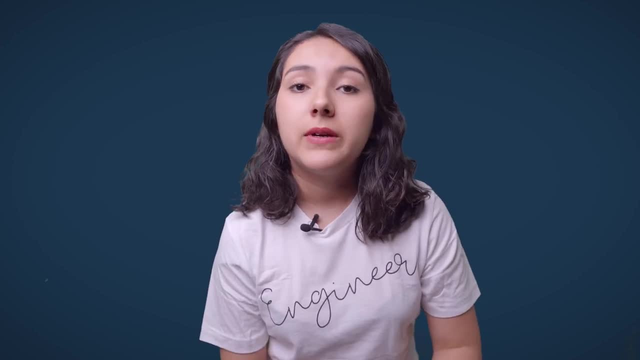 fall off. So it's better to make sure that you have your occasionally in-grass locked device in place and Command be careful if you want to. before you visit them, fact check using a 10-day pain vaccination. The next real regulatory pathway that we're going to be talking about is 510k. 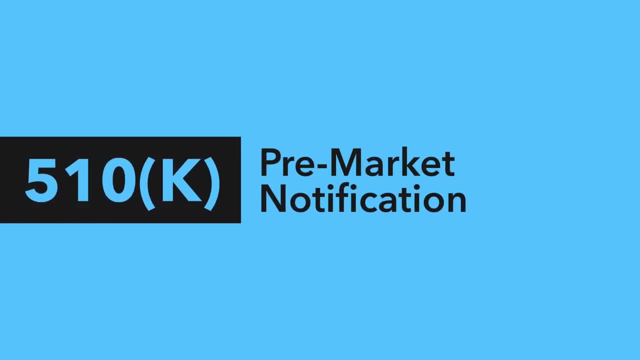 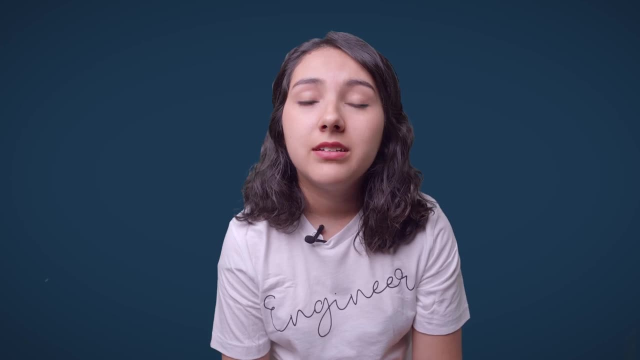 510k's are also known as pre-market notifications. What I want to say is that these are the most commonly used. Now, the thing about getting in a 510k is that you need to have what is called a predicate device. A predicate device is really a device that gives a pre-market prediction. 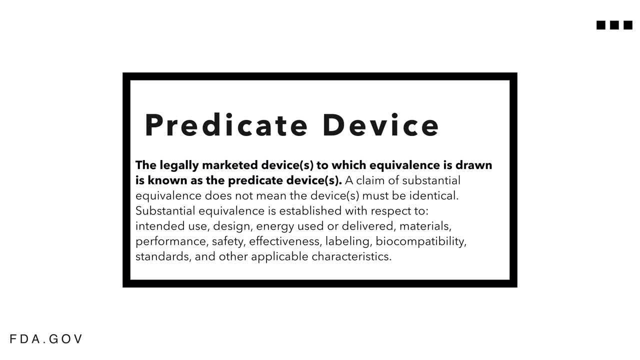 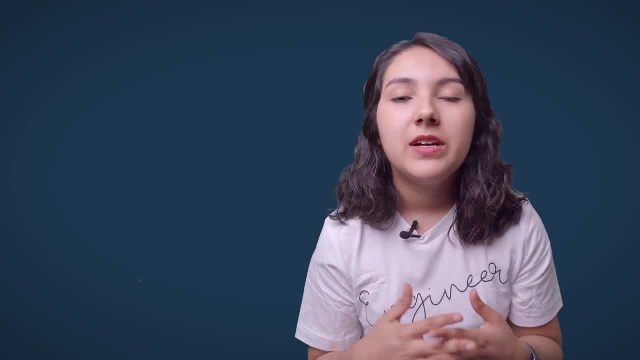 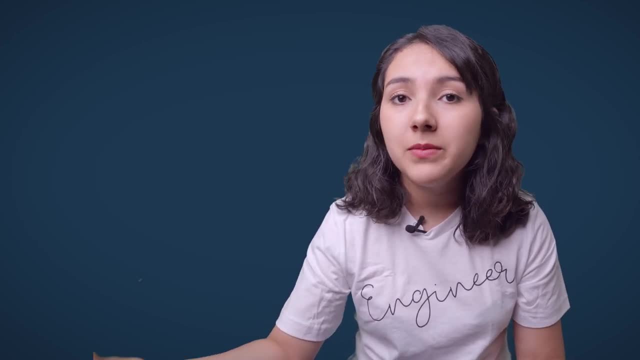 definition a device that is already legally marketed in the us and that you can use as a comparison for your new device. so, for example, if i have a device that i want to put in the market and there's already a device that's very similar to it already being legally sold in the market, 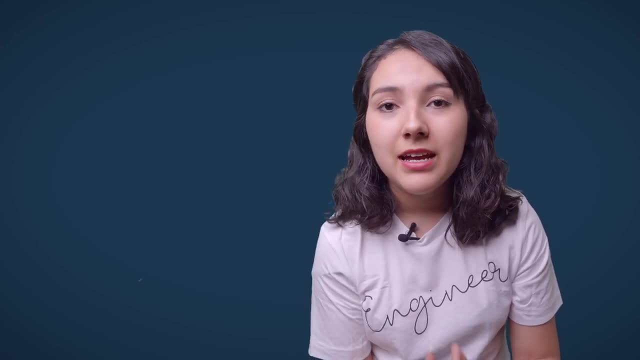 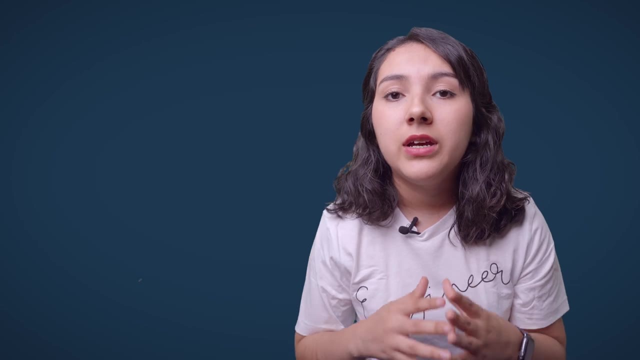 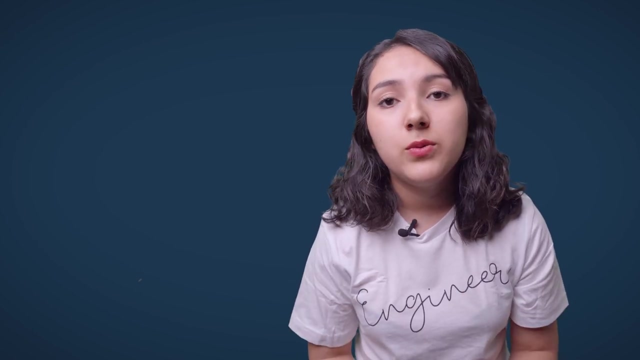 then i can apply with a 510k saying: hey, my device is very similar to this other device that is already approved, so that way you can use the data that supports that device to support your device. the only thing that you have to do with the 510k is provide proof that your device is substantially. 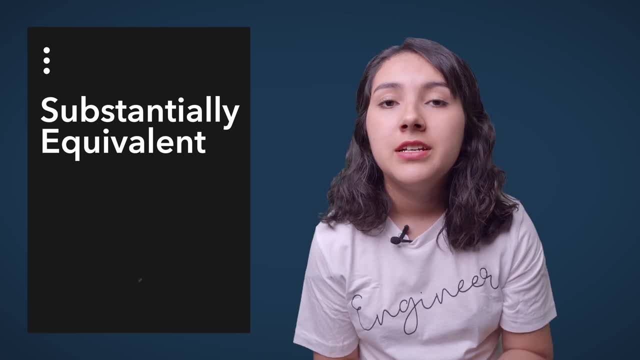 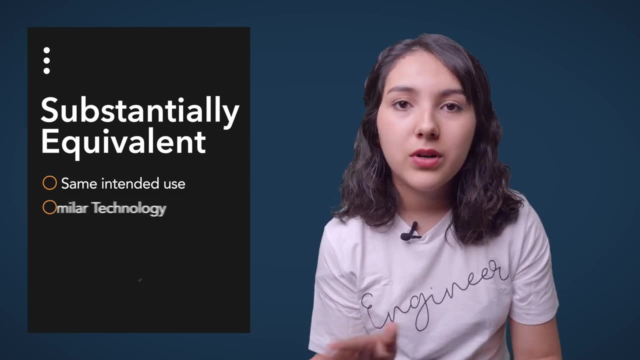 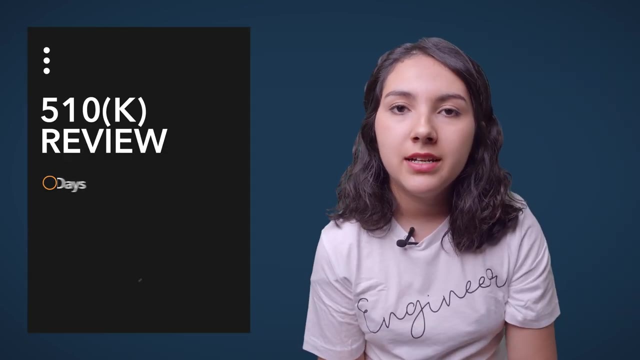 equivalent and a device is considered substantially equivalent if it has the same intended use and if it and if its technological characteristics are very similar to the predicate device. the fda takes up to 90 days to review your 510k application and if your device is determined to be. 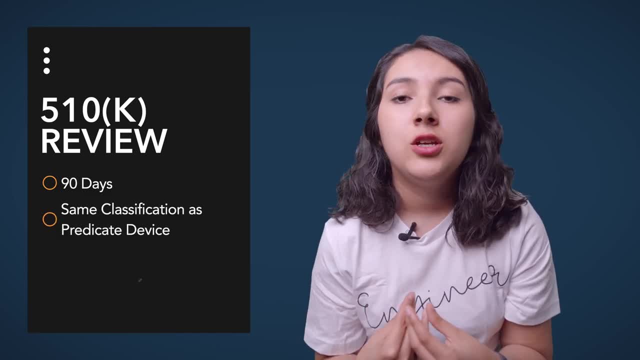 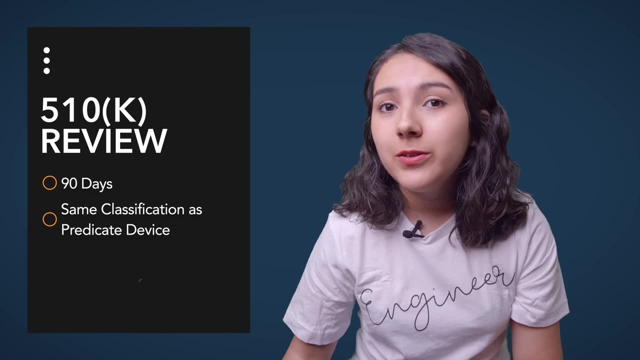 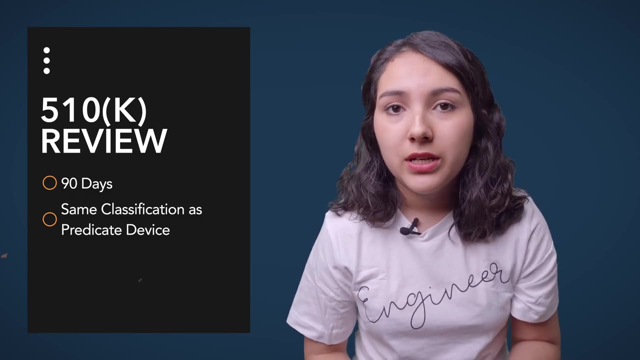 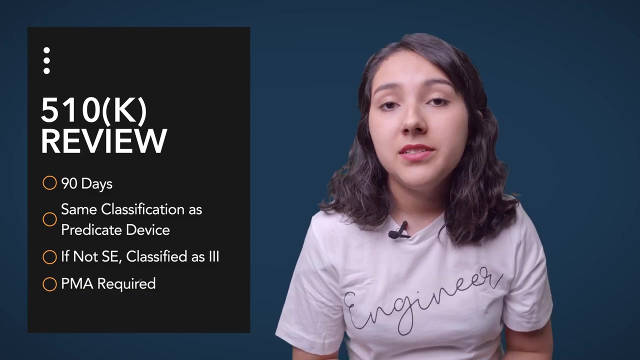 substantially equivalent to the predicate device, then your device gets classified with the same class number that the predicate device has. however, if your device is not really considered substantially equivalent to the predicate device by the fda, then you would get placed into a class 3 classification, which means that you would have to get a pma. some examples of class 2 devices that: 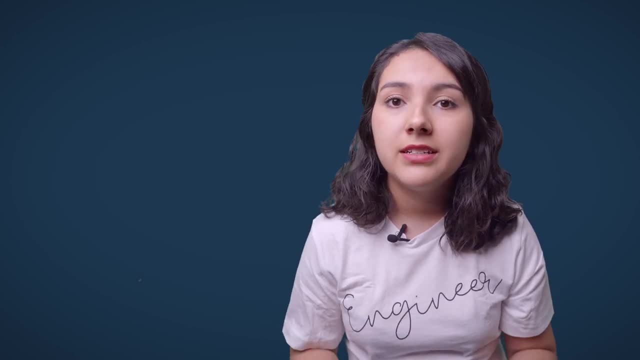 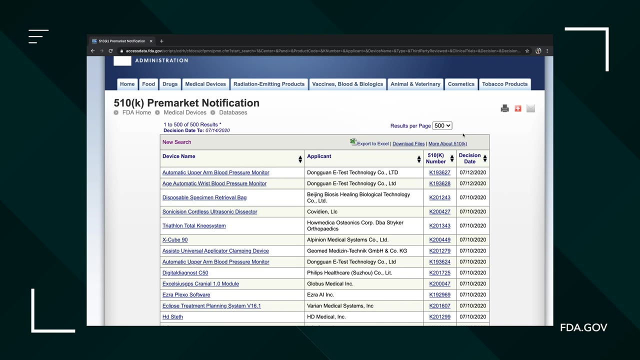 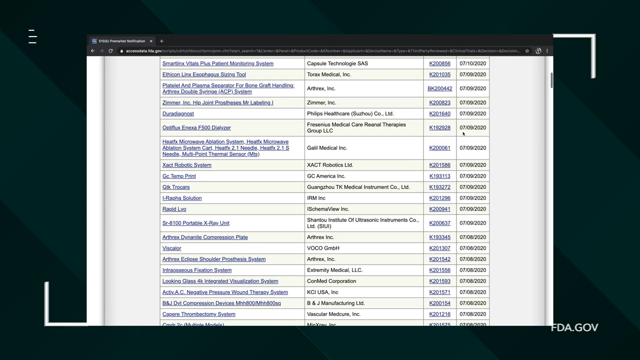 have 510k clearances include fetal monitors, dialysis machines and x-rays machines, and something that i think is really cool is that fda actually has a database where you can go and see of all the 510k applications that have been cleared by the fda. so next comes a pma or a pre-market. 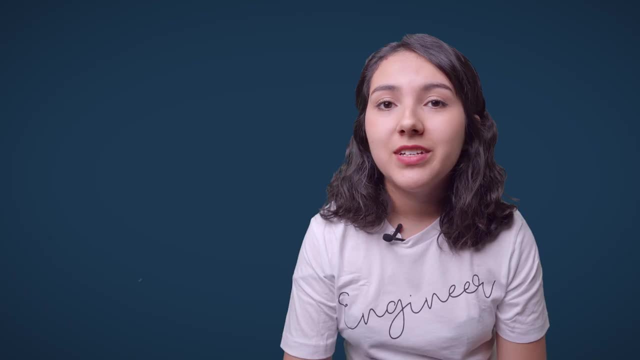 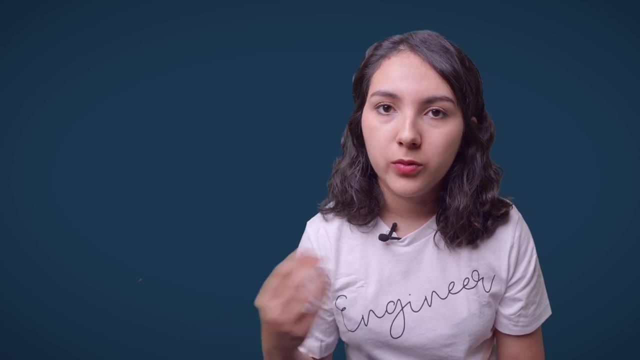 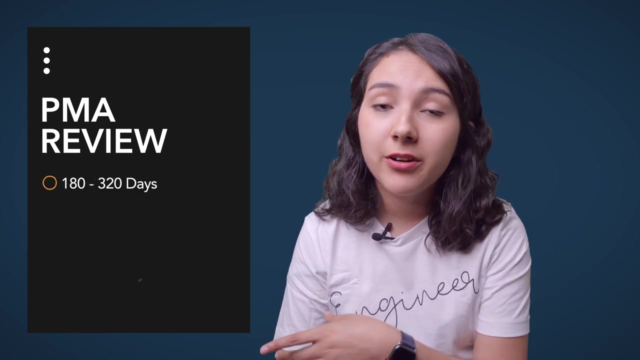 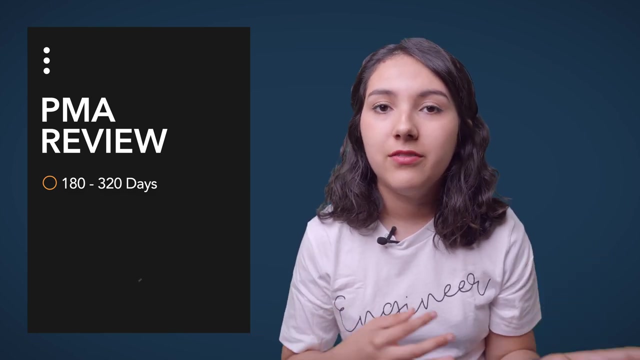 device. pmas are the most intense review processes or regulatory pathways that a device will follow to get approval to be sold in the market. fda reviews for pmas usually take anywhere between 180 to 320 days. so for the fda to determine that a class 3 device is safe and effective, 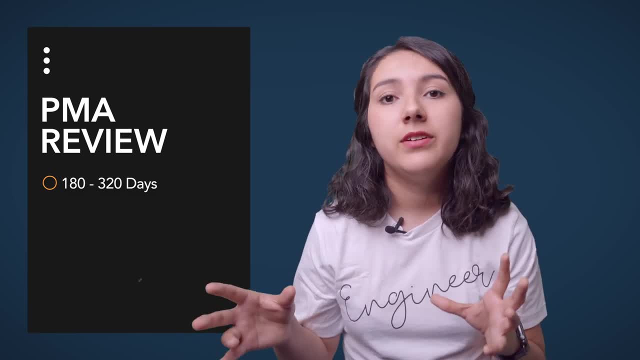 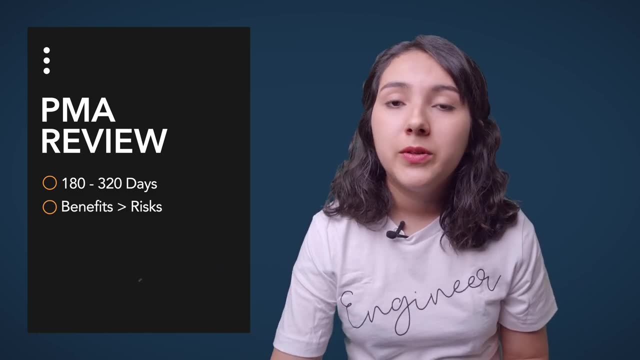 it must first conclude that the potential benefits of this new device completely outweigh the many risks that it could have. another thing that you must prove in a pma is that your device will help a large portion of your target population. and the third concept that you're 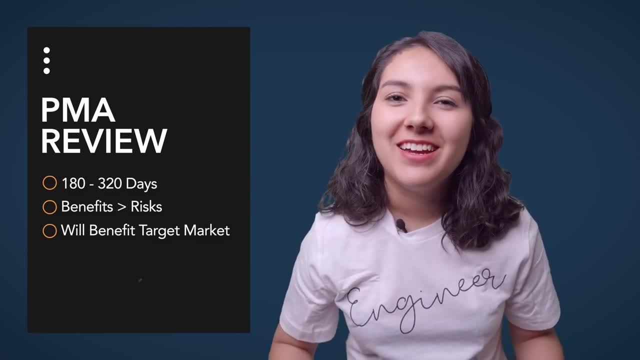 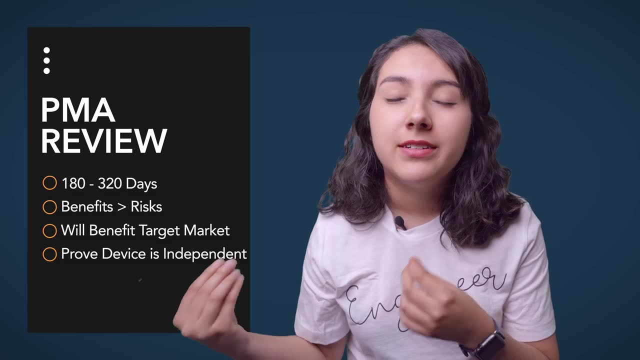 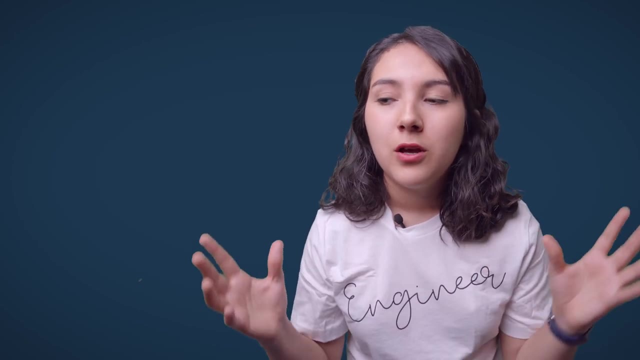 really trying to prove using a pma is that your device is independent, which means that you're not using other devices data to support your own. and that's really what the fda is trying to see: that your device is not safe and effective. so the fda is using a device that is novel and it's safe and effective, so it actually involves a. 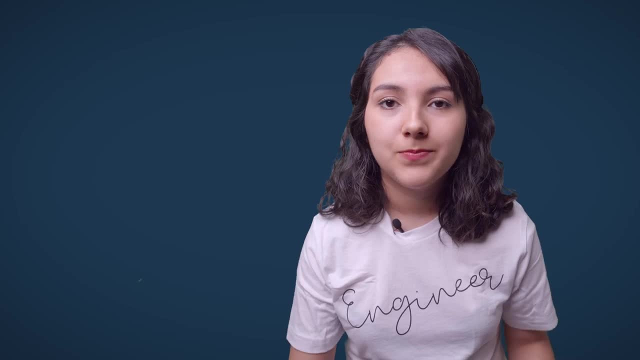 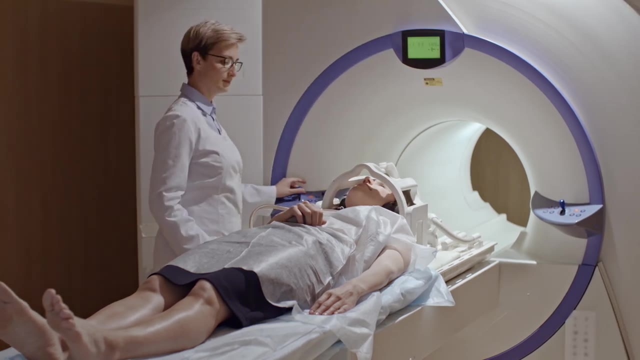 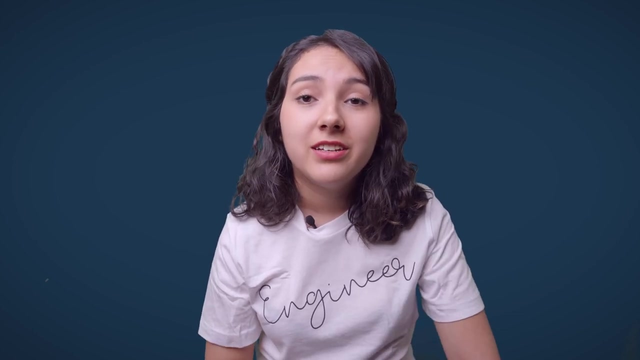 lot of non-clinical and clinical testing in your review process. class 3 devices include a lot of implantable devices like pacemakers or defibrillators and also like digital mammography devices, and the last regulatory pathway that we're going to be talking about is actually one that i 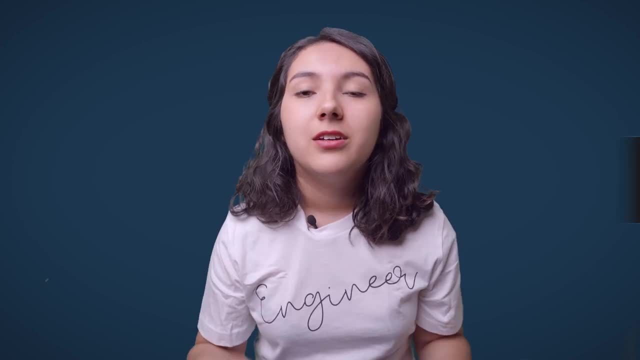 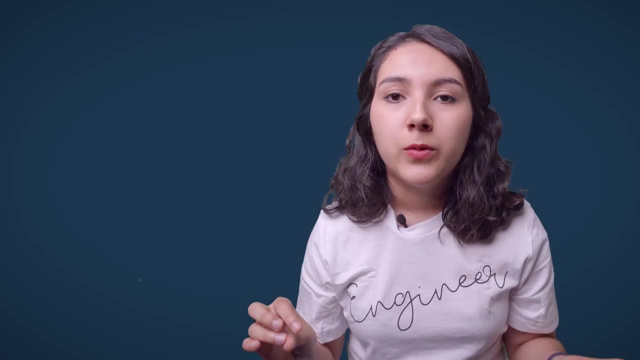 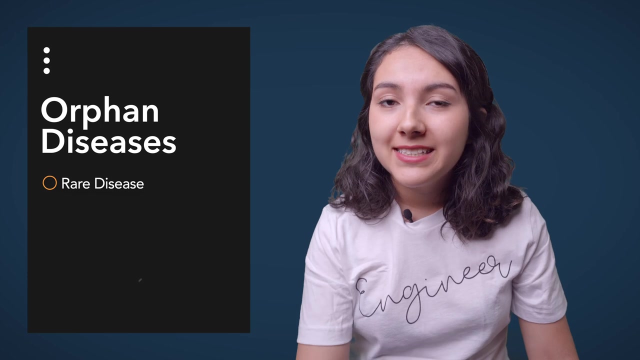 think is really interesting and it's also not very common. it's called a humanitarian device exemption and this regulatory pathway is used for when coming up with devices for orphan diseases. what are orphan diseases? orphan diseases are rare diseases that have less than 200 000 conditions. 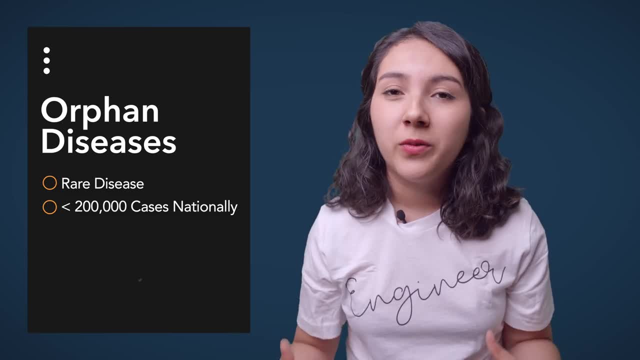 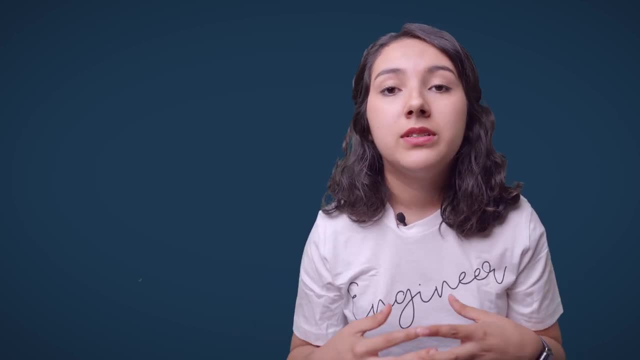 in the nation. usually these diseases are so rare that they're really hard to study. this is why the fda created an act that would let companies come up with devices to treat these without having to have a large scientific knowledge of the disease to be used in their device. and then the fda is. 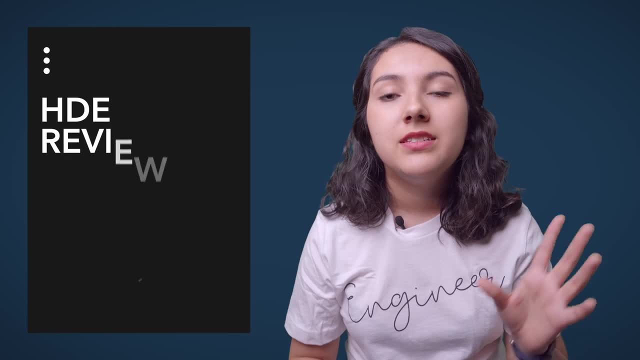 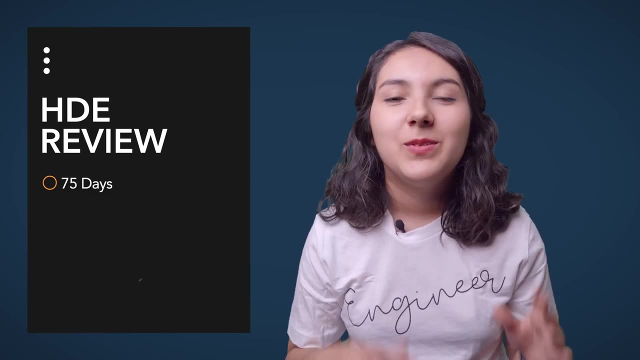 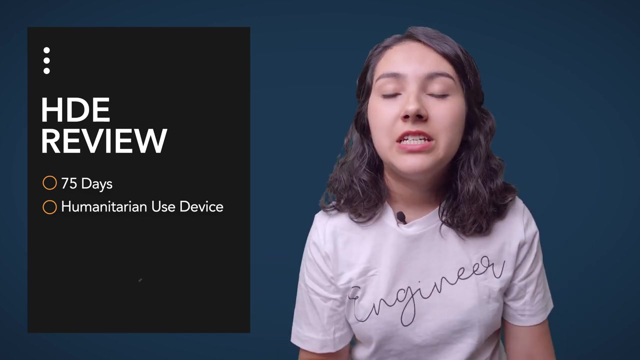 scientific review of them. So to review a humanitarian device exemption it'll last about 75 days, so it is the shorter pathway that any device could take. So with this application you get what is called a humanitarian use device or a HUD. So to make an HCE you really have to prove that there are no other similar. 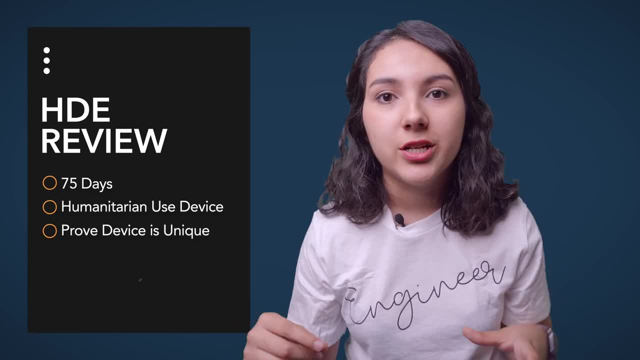 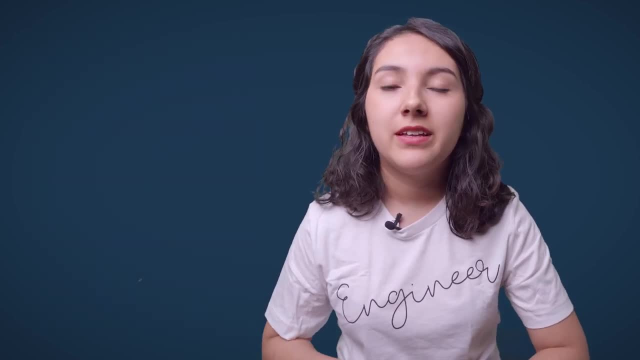 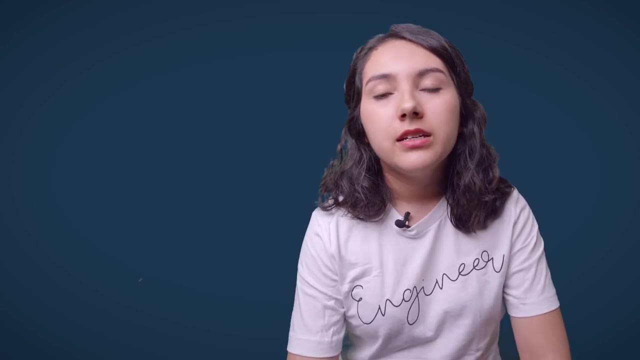 devices that could help your cost or disease that you're trying to treat or diagnose already legally being marketed. So these are all the regulatory pathways that the FDA uses to control the approval or clearance of medical devices into the market, and I think it's really important to learn about this, because it's not really something that you see. 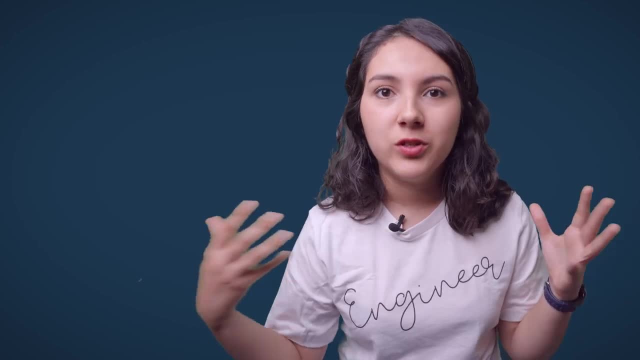 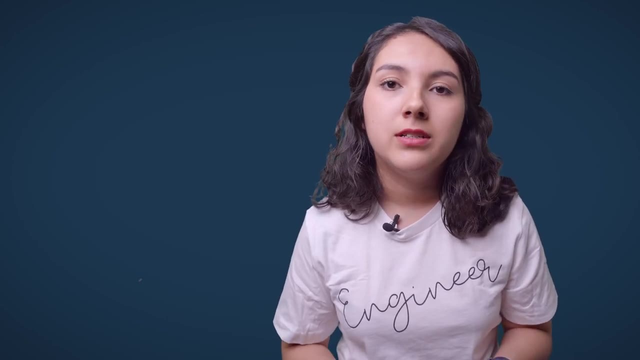 much of in school. I mean, I get it. we're biomedical engineers, so we need to learn about, well, the other side. you know making the technology, But I think it's also very important to keep an open mind and learn about what it takes to even put that device in the market. 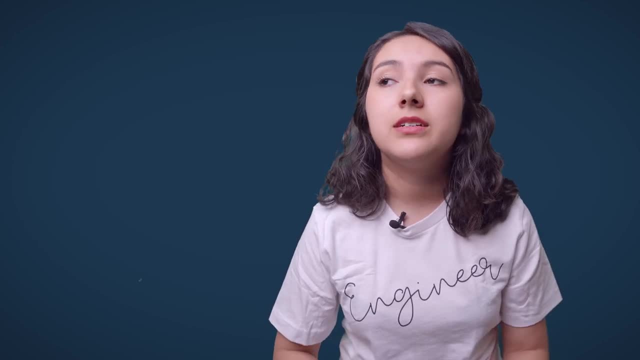 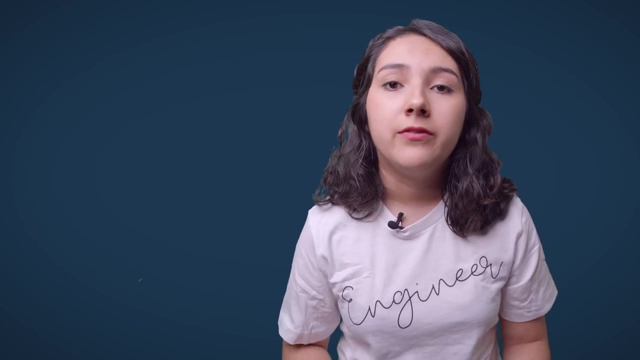 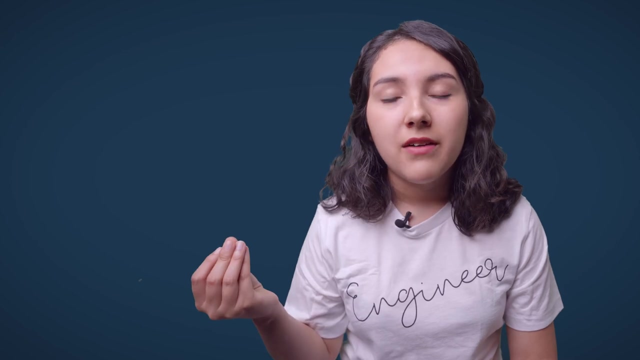 It's very important to know about the different regulations, because there are so many medical devices or kinds of them, and I think it's especially important if you're either working on a startup or if you're thinking of creating your own company. It's one thing to have a great idea. 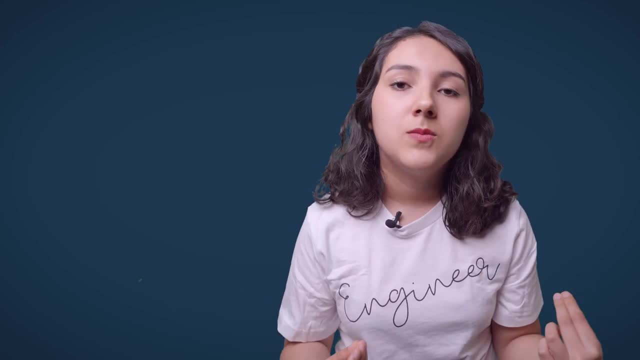 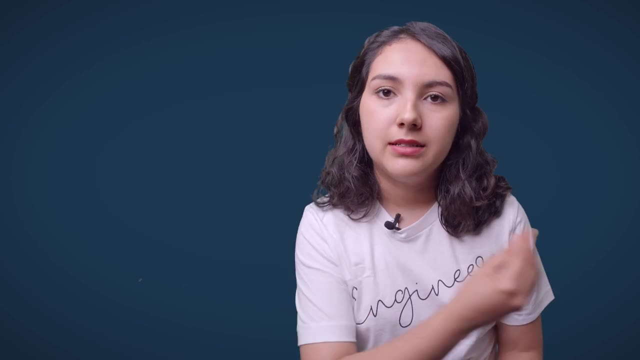 but it's a whole other thing to create a business model, and then it's a whole other thing to know how to. how are you gonna get it right? I think those three things are the holy trinity of medical devices, and we really want to start this series. 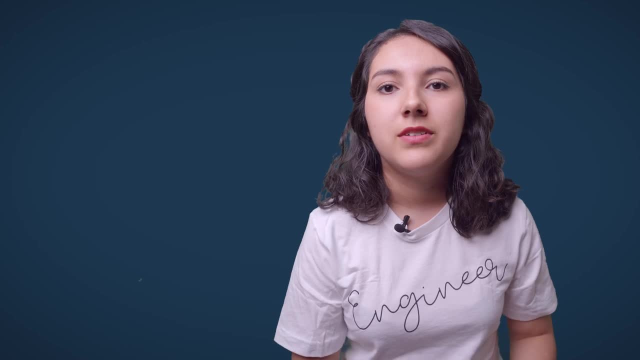 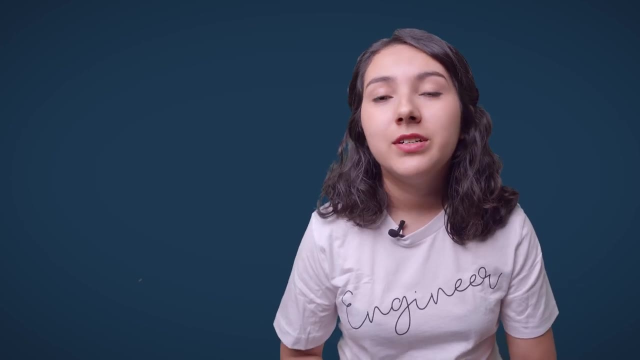 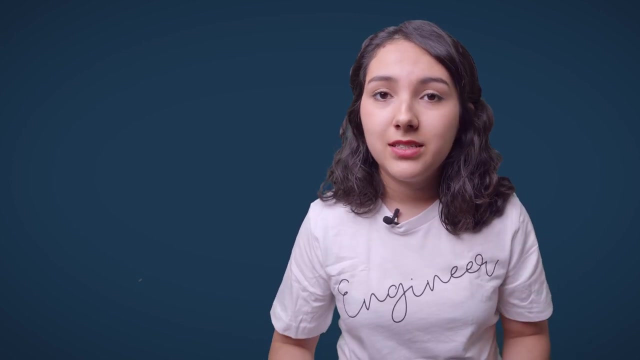 focusing on the regulatory side of medical devices and other things, because the FDA also regulates pharmaceuticals and combination devices. But we also want to continue this series talking about just regulatory stuff and maybe going more in depth. for example, and what it takes to have a 510K application, what it takes to 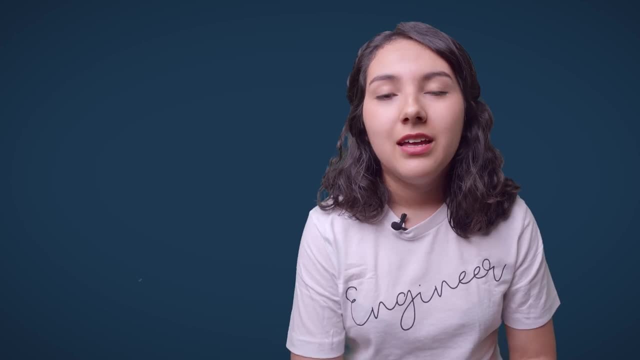 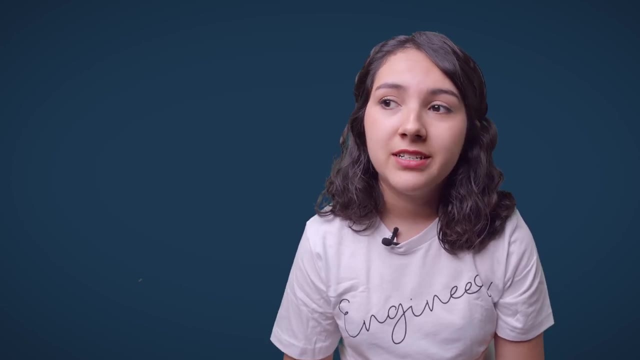 submit it to the FDA, how you even do that in the first place, and just about any other regulatory pathways as well. And just a little reminder that all this information is in the FDA. FDA does such a great job of putting together all this information in their website. 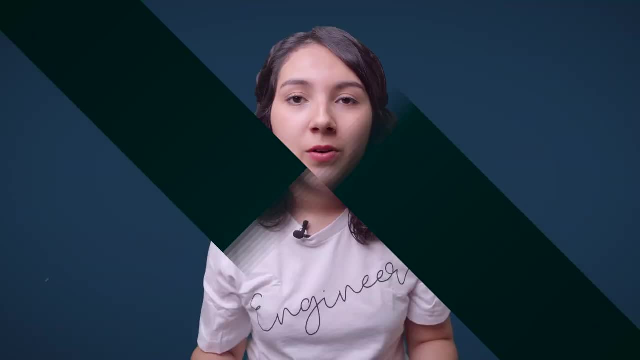 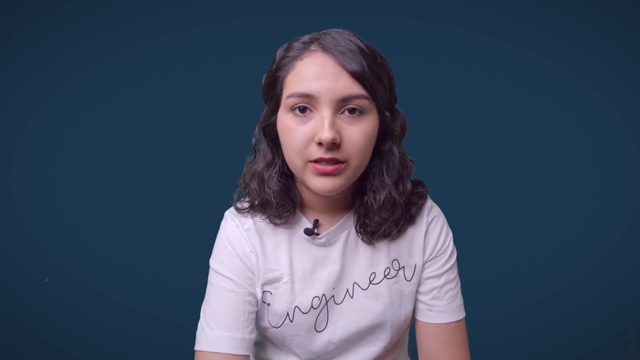 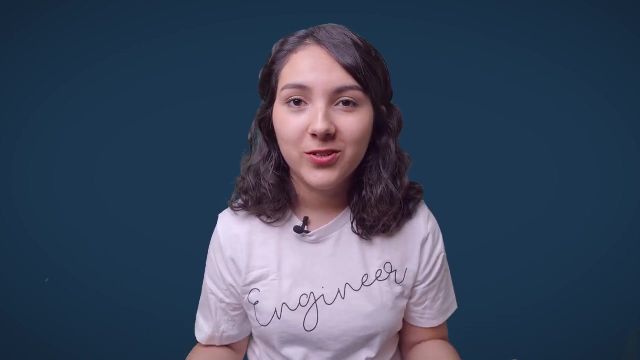 and I really love how they organize all you have to know. So if you're ever curious, just go visit their website and there's a lot of information on how they regulate medical devices. Thank you all For watching this. let us know if you enjoyed it and I really hope you learned something, and there are actually a lot of.